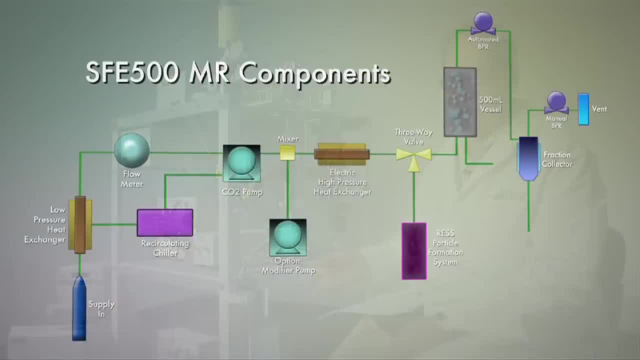 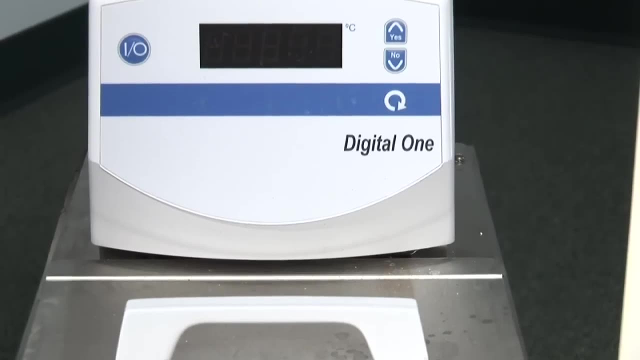 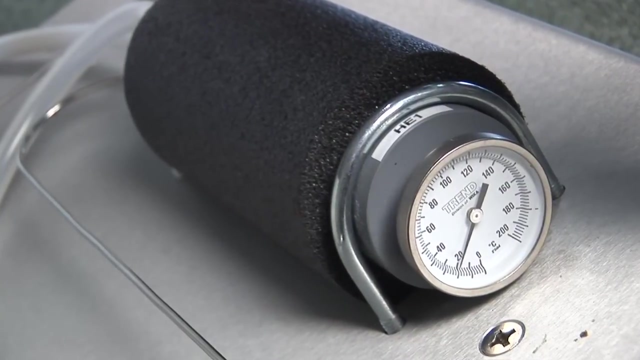 extracting thermally labile compounds from natural products. Components of the extraction system include the recirculating chiller. This provides chilled ethylene glycol solution to the heat exchanger. The heat exchanger cools the CO2 before it goes to the pump. 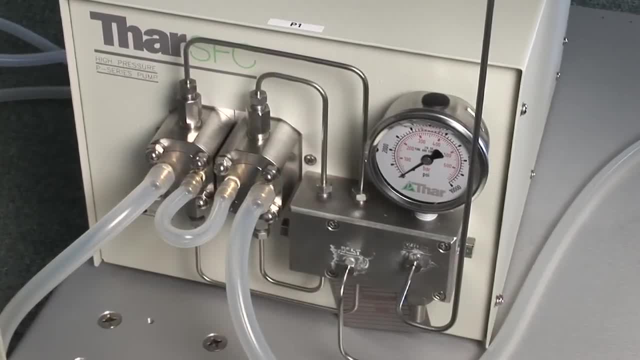 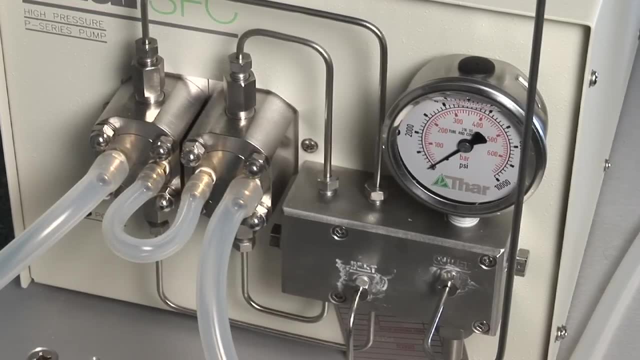 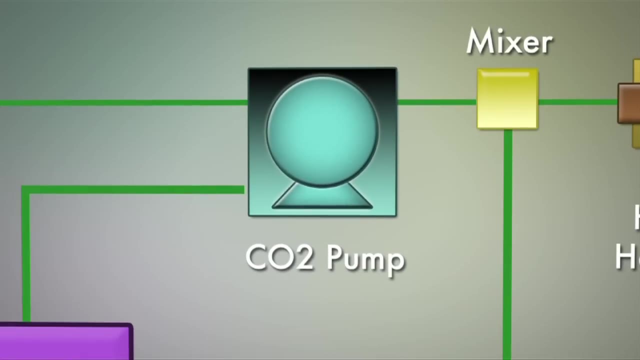 When the CO2 reaches the pump. it is a liquid Allowing the pump to deliver denser CO2 and it cools the pump, reducing pump head cavitation. Its maximum flow capacity is 50 ml minute of liquid CO2.. This high pressure CO2 can 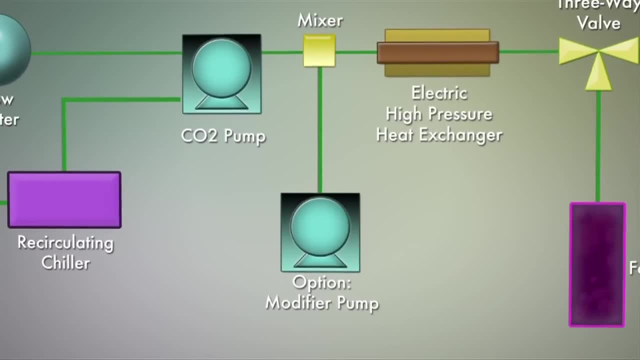 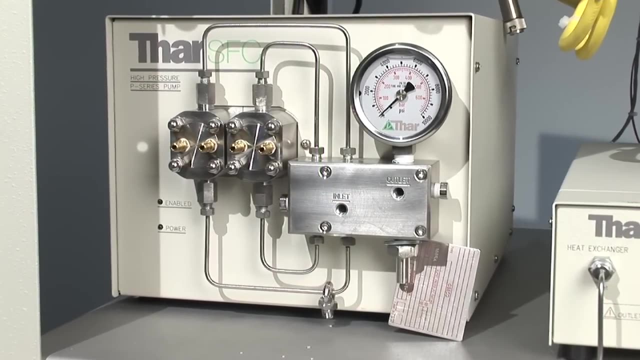 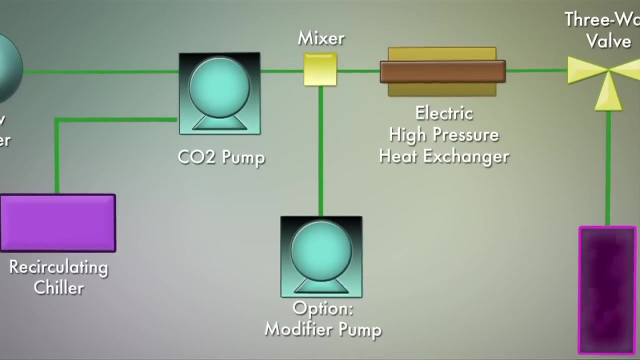 then be mixed with a co-solvent, sometimes called a modifier, And typically that's added in amounts of 3 to 5% from this modifier pump. The modifier can be any organic solvent. The mixed solvents- CO2 and co-solvent- are then sent to a second heat exchanger And in this 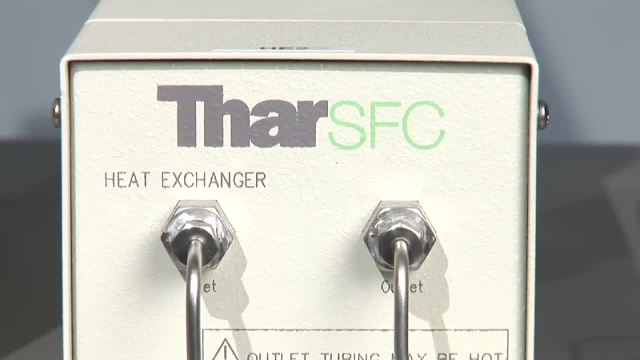 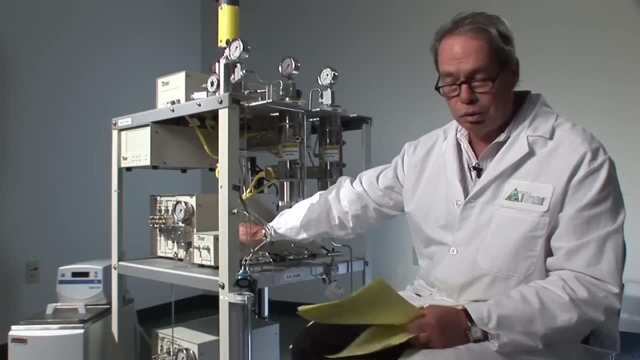 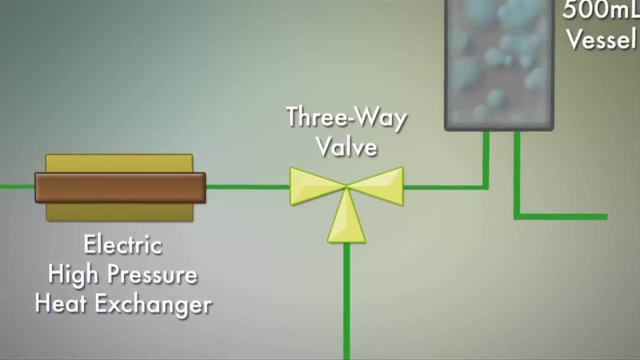 heat exchanger. we heat the mixture of CO2 and solvent up above 31 degrees centigrade, So it is above supercritical conditions and we now have a supercritical fluid. The mixed solvent leaves the second warming heat exchanger and goes into a three-way valve. 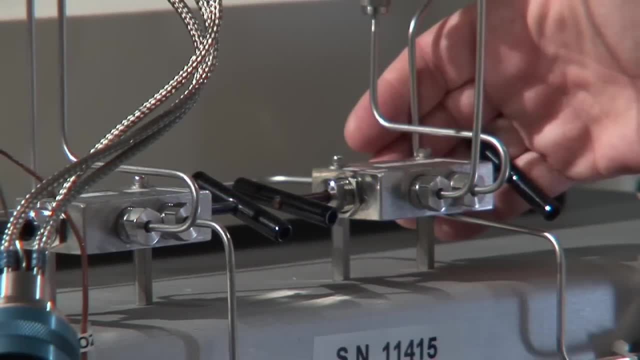 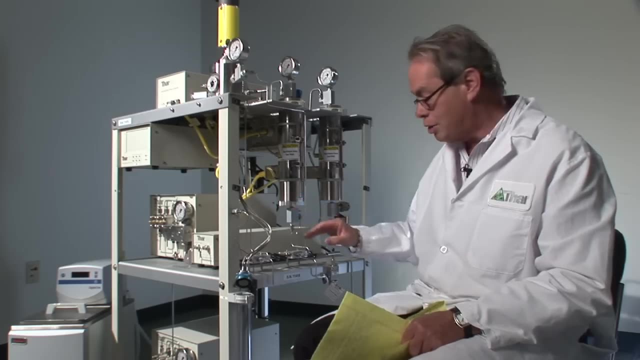 The three-way valve can direct the flow either to the main pump or the technical removal of the metal. So it's a very high pressure, high flow for any part of the process. This the solvent extraction system or the particle formation system, When we're using it in the extraction mode. 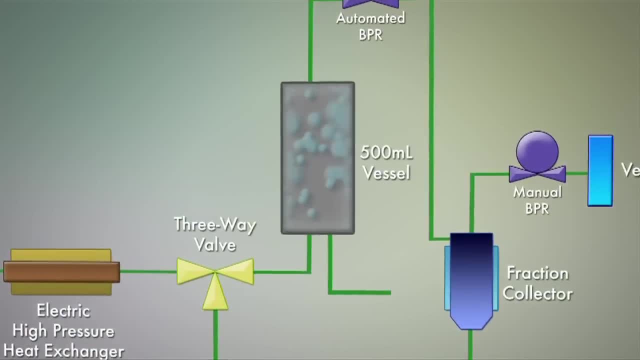 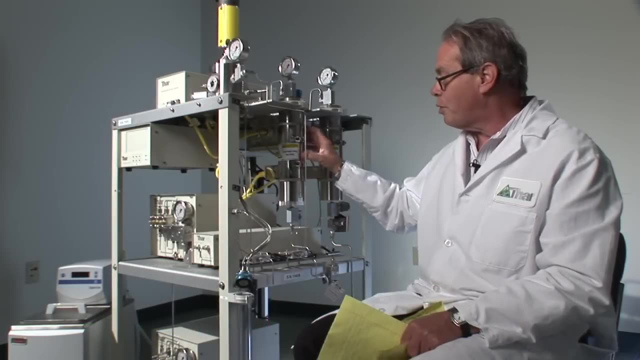 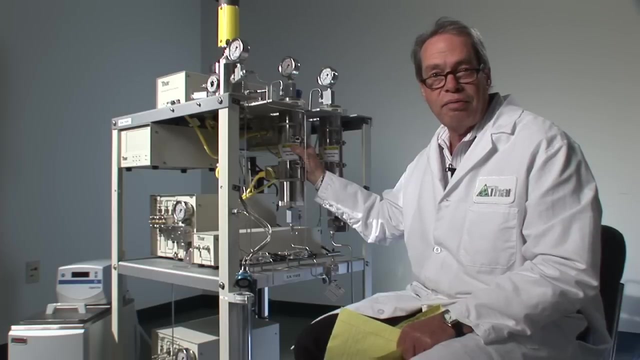 the flow is directed toward the bottom of this 500 mL extraction vessel. The CO2 flows in through the bottom of the extraction vessel, flowing up through whatever it is the extraction vessel contains. It dissolves some of those components- maybe caffeine from coffee beans. 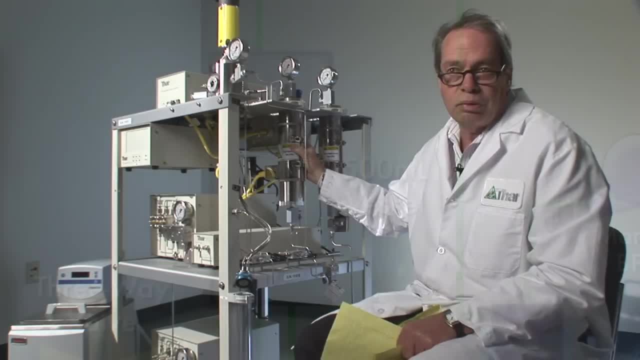 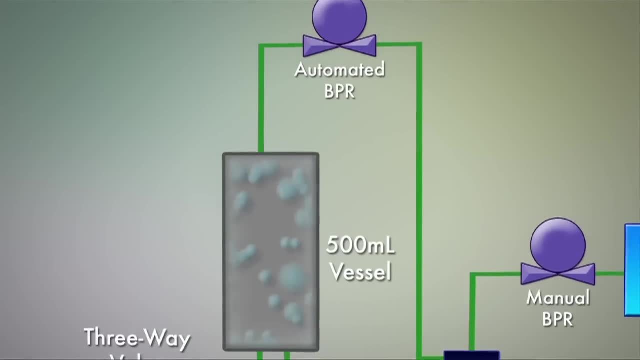 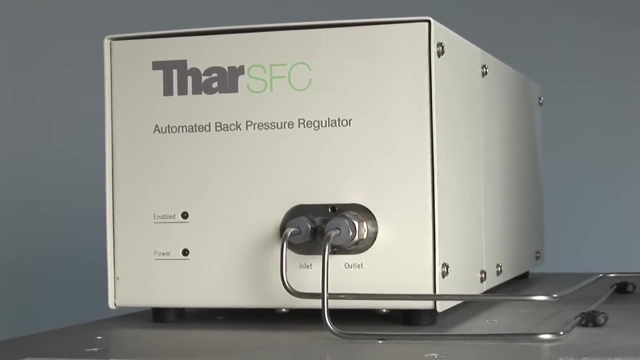 maybe some drugs to be tested from plants from the Amazon. The dissolved components and the flowing solvent leave the top of the extraction vessel and go into the back pressure regulator. The pressure is reduced to about 3 bar. Now it turns out that the solvation power of a supercritical fluid